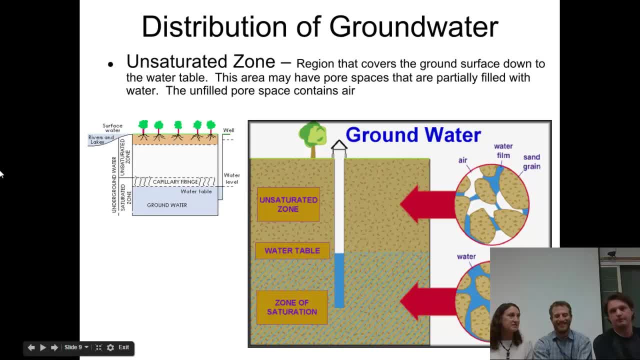 Okay, so we're going to start to dig in on some of the basics And the basic terminology about groundwater And we're going to start with the different zones under the ground. So we have to try to think about what's under our feet and what we know about that. 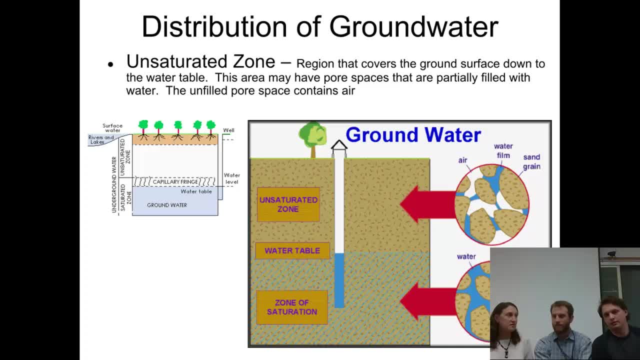 We're going to start with the first zone being either called the unsaturated zone or the zone of aeration, And I kind of like to remember that it is called the zone of aeration because that helps me remember that the pores in between the unconsolidated sediment. 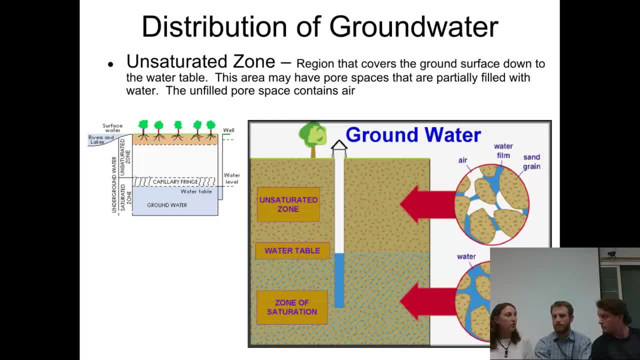 or the pores in between soil grains are full of air And or water, But they're not fully saturated with water in that zone, right, Okay? So as we move further down, at the end of the unsaturated zone we run into something called the water table. 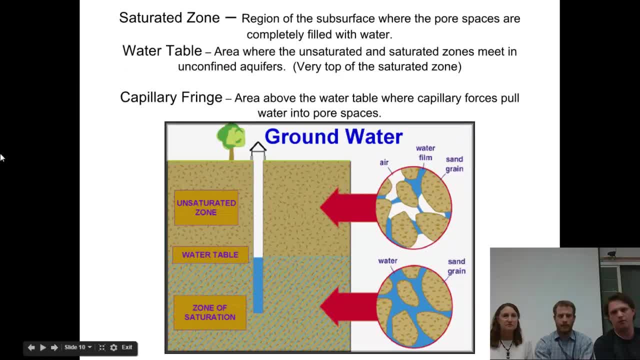 So with the water table, this is where you dig down and essentially you're hitting water. So if you were to dig a while or like, I think, when I was digging at the beach, like last weekend, because I still do stuff like that- 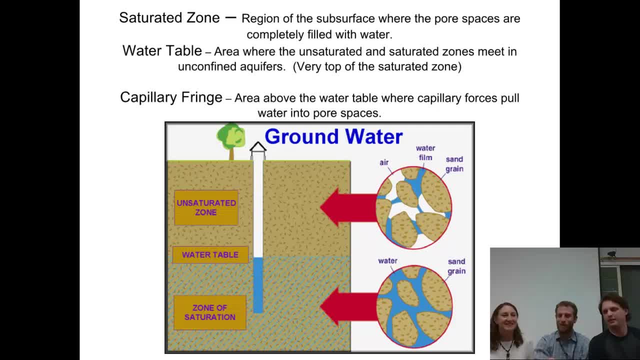 It was snowing, But you dig a hole and as soon as you hit water, that's the water table right. And so what's going on with the pore spaces there? Well, the pore spaces at the water table begin to be filled with water. 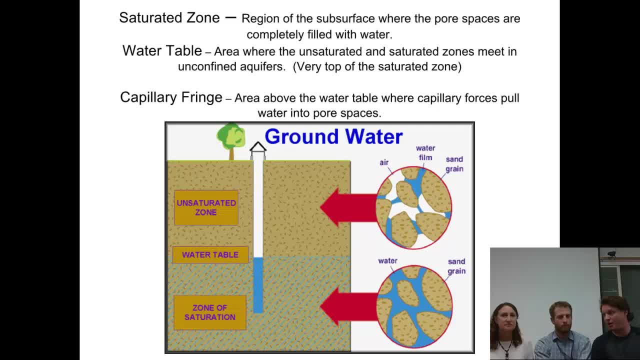 And then everywhere below that water table we're going to call the saturated zone, And if we think of something as saturated, or a sponge or something like that, that's saturated, It's full of water. So all the pore spaces in the saturated zone are full of water. 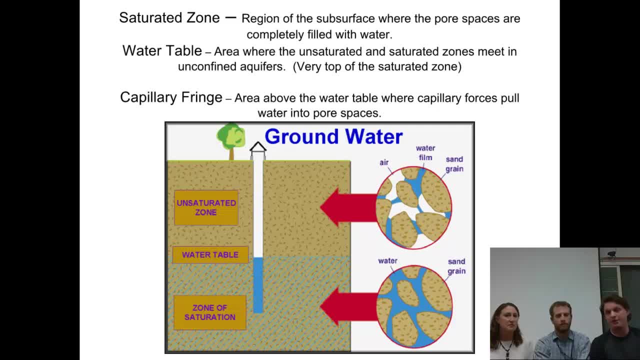 And the water table marks the height of the zone of saturation. At that interface between the unsaturated zone and the saturated zone at the water table, we have this little area called the capillary fringe. So the way I like to think about it is: if you take a paper towel and you just dip it into water, water gets sucked up into the paper towel. 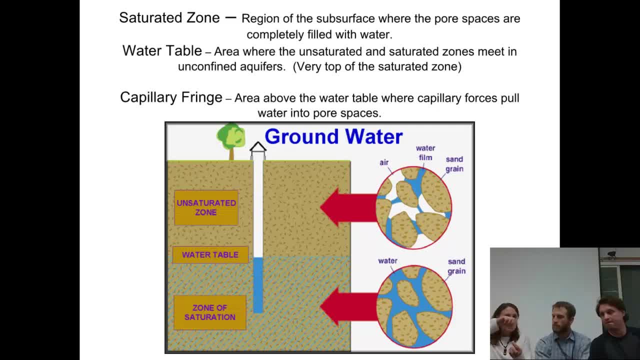 And that's a similar situation with the capillary fringe, where you have little bits of water being sucked up into the pores in the unsaturated zone at the top of the water table. Right, Okay, So we've got the unsaturated zone on top where the pores are filled with air and or water. 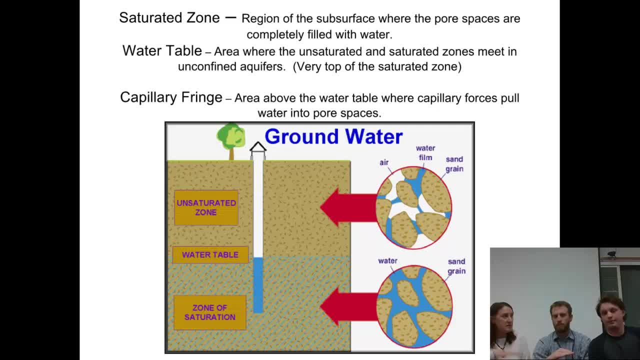 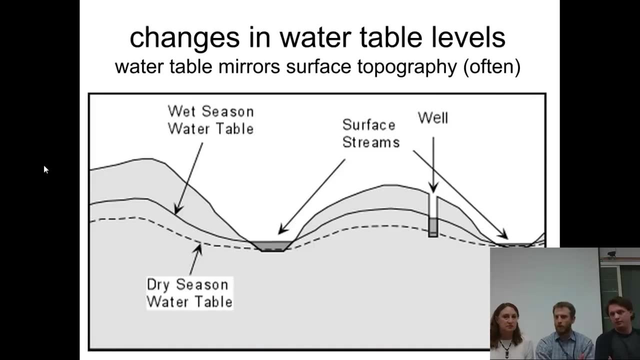 We have the water table that separates that unsaturated zone from the saturated zone, where the pores are full of water, And the capillary fringe at the top of the water table. Okay, good, Let's go on. So if we take a look, the water table, for the most part, is going to basically mirror what the topography looks like at the surface. 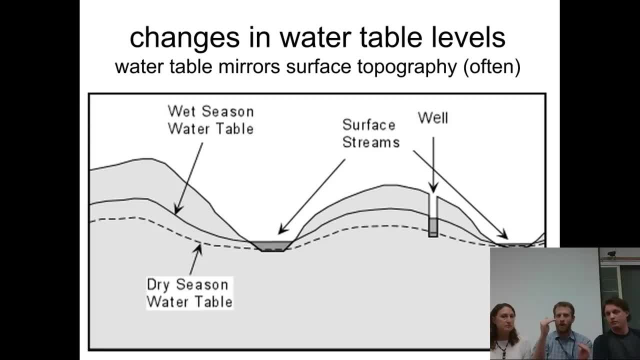 If you've got a higher point in elevation, Like a hill or a mountain, your water table is going to somewhat mimic that, So it's going to take the same shape. So if you look at the picture there, they've got the wet season water table and the dry season water table. 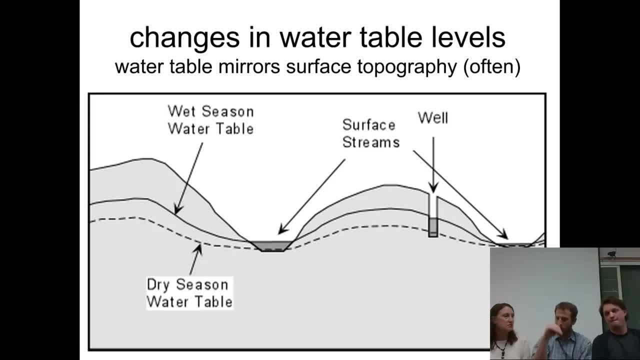 Dry in the dashed line and the solid line for wet. it kind of takes the same shape of those hills there. Okay, So I'm guessing we have to be careful of that variation between the wet and the dry season when we start to talk about wells. 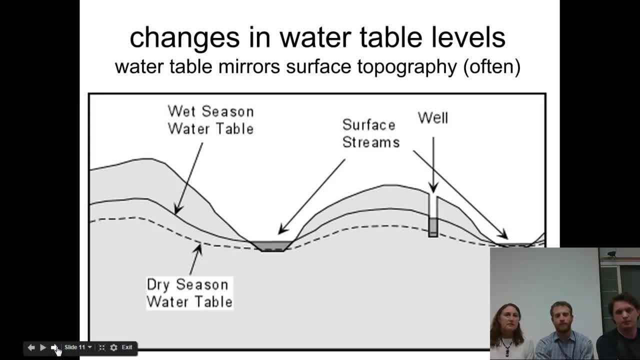 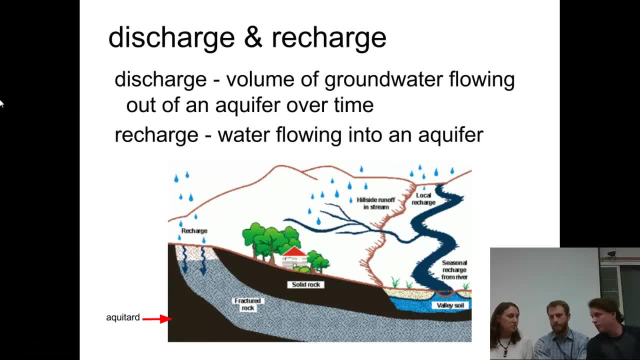 Mm-hmm, Mm-hmm, Now thinking about how the water gets into this saturated zone, and actually we haven't given the saturated zone a name yet. Yeah, So we've got the unsaturated zone, the water table, the saturated zone, and this saturated zone has a name, and it's called an aquifer right. 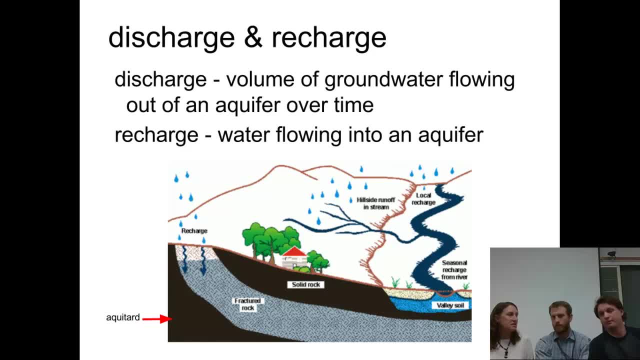 So we have water flowing through this aquifer. Well, how does it get into the aquifer? And there are a couple of ways that water can get into it or recharge an aquifer. One of the ways, simple way, is rain or snow. 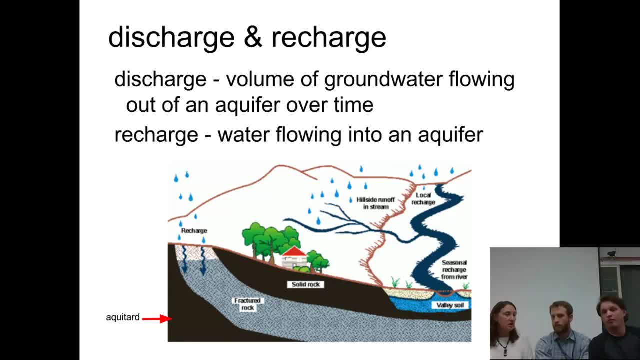 Snow falls on the surface, soaks through the soil layer, the unsaturated zone, makes its way down into the saturated zone and recharges the water in the aquifer. What are other ways You can have melting snow? Okay, So like right now, it's winter by us and all the snow is starting to melt. some of that water, as it melts, infiltrates into the soil. it recharges some of the aquifer. 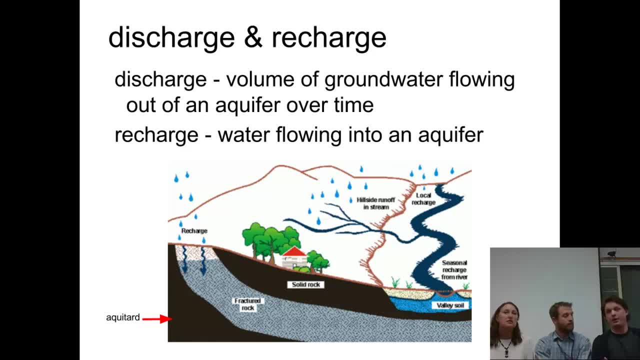 Okay, and then water flowing out of the aquifer Would be like a river, So we can see, or we can see a river. A river that would be flowing would also be taking groundwater out of the system, and then also pumping water out of a well could also be taking water out of the system.